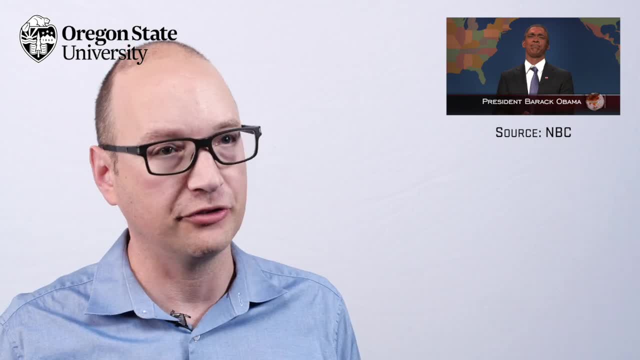 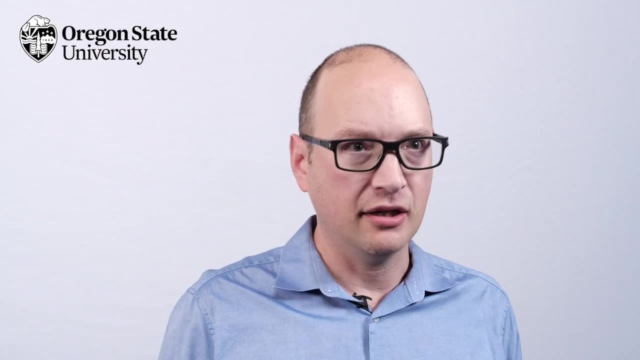 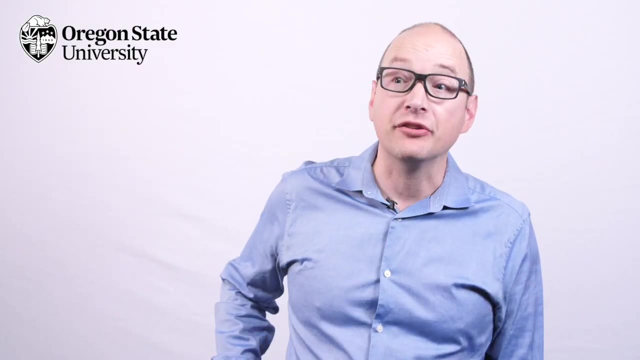 in a relatively gentle way in which everyone is in on the joke together, including the person being caricatured. Juvenal satire tends to be more bitter and dark, expressing anger and outrage at the state of the world. A famous example of Juvenal satire is by another 18th century writer, Jonathan Swift. 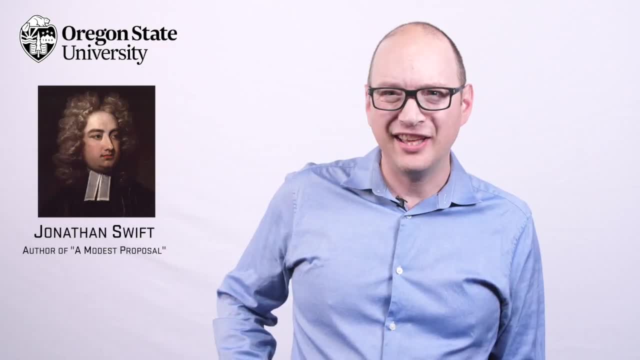 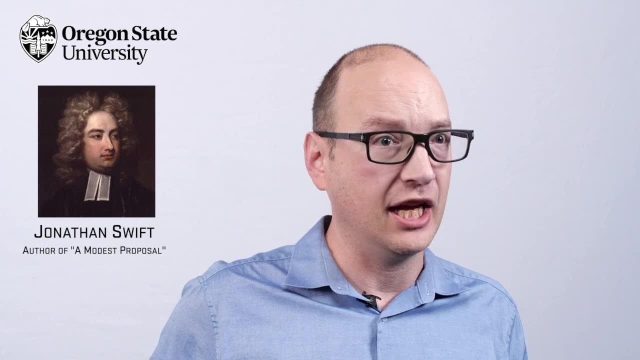 His A Modest Proposal is a prose pamphlet that initially appears to be a serious, well-intentioned attempt to suggest a solution to what was a major problem at the time- the impoverished state of Ireland- due in no small part to absentee English landlords. 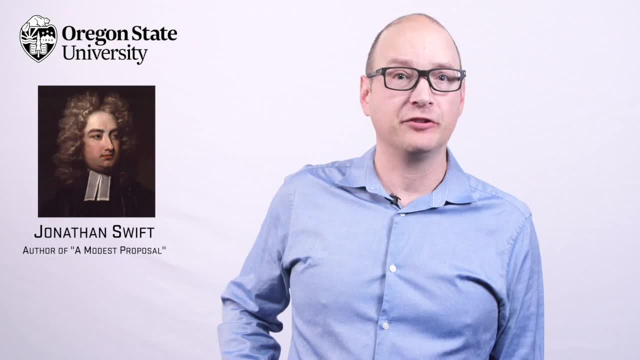 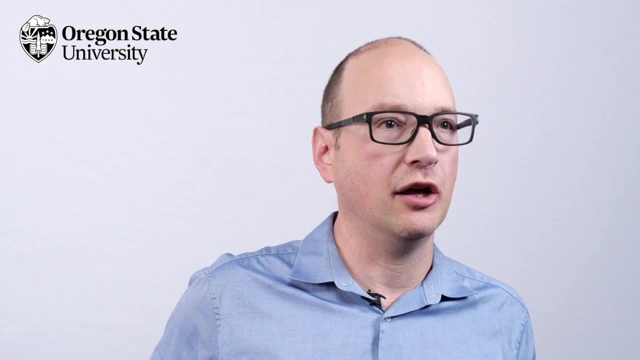 who owned a lot of Irish land but reinvested very little of the profits back into the Irish economy. As the narrator begins to explain his plan to invigorate the Irish economy and make all the poor Irish families useful again, however, the reader slowly begins to see that the narrator's proposal 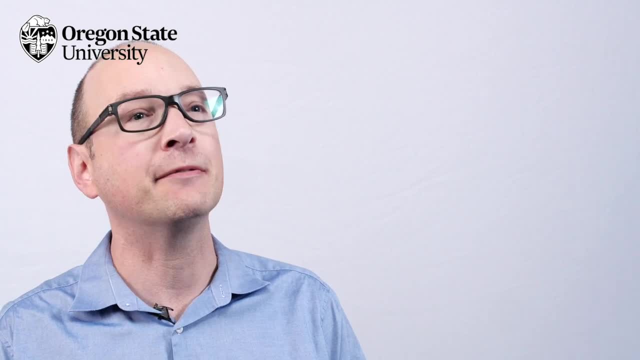 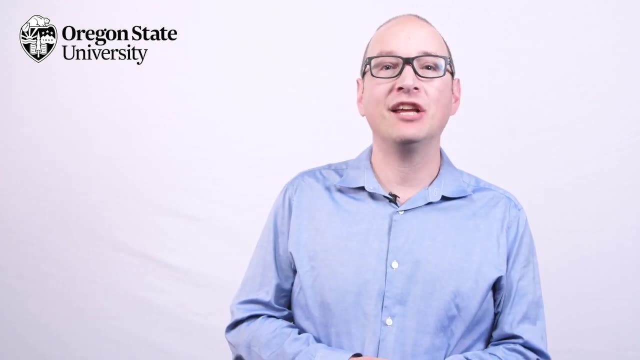 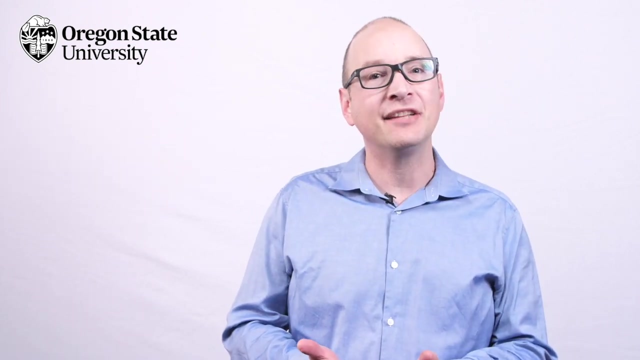 is actually for Irish women to sell their babies to be eaten by their Anglo-Irish landlords. A Modest Proposal is thus an angry denunciation not just of the rapaciousness of the English and their lack of care for their Irish tenants, but also of the kind of bureaucratic mindset 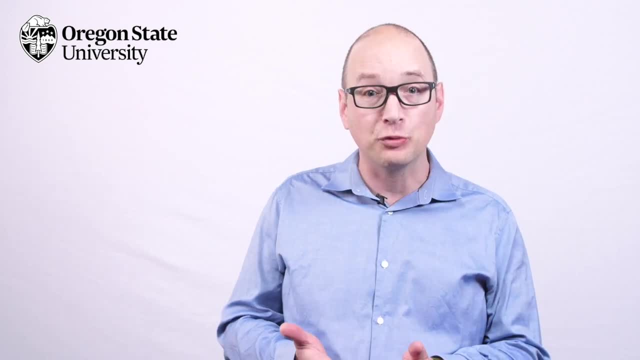 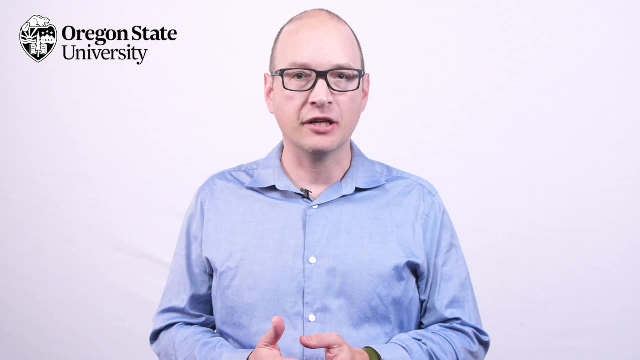 that becomes so enamored with its own problem-solving that it forgets that real humans will be affected by its plans. A modern example of Juvenalian satire would be the parodies of contemporary advertising done by groups like Adbusters, in which they peel away the shiny. 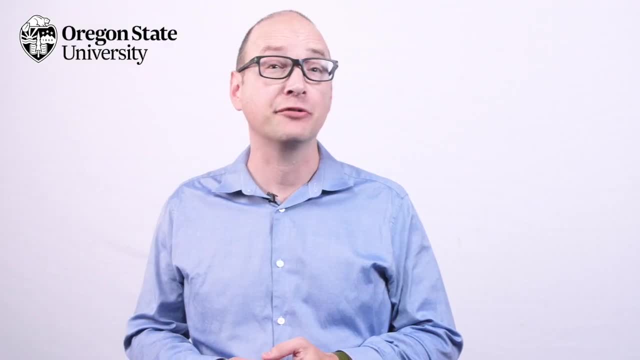 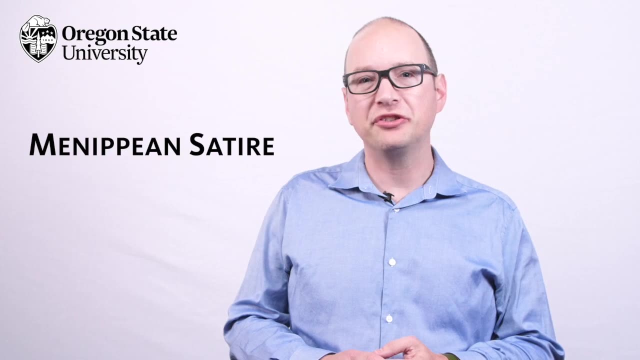 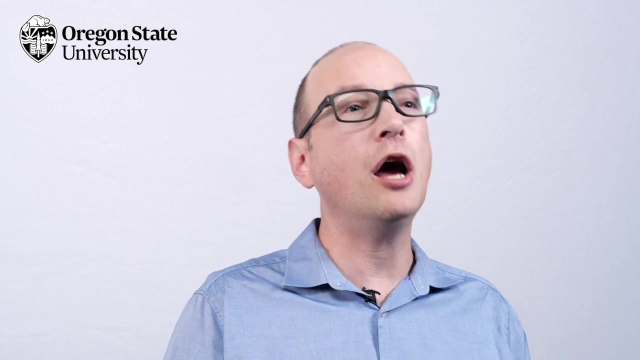 veneer of advertising, to show the heartless greed that lies underneath a lot of corporate capitalism. Finally, there's Manipian satire, Reserved for prose works that still resemble that original connotation of satire as a miscellany or containing multitudes. A canonical example of the Manipian satire is Lawrence Stern's. 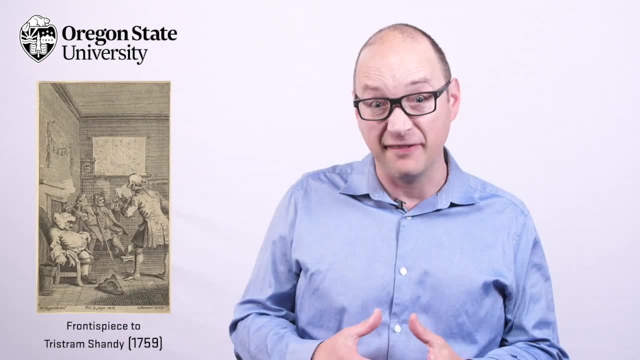 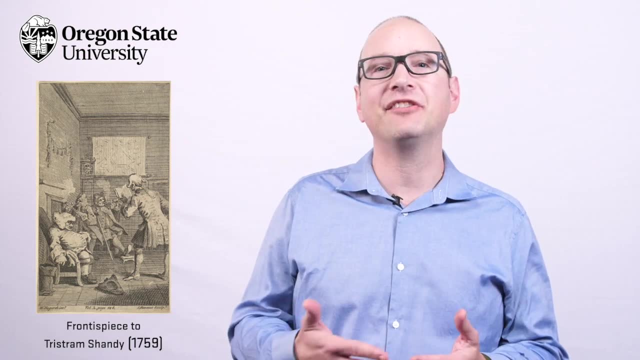 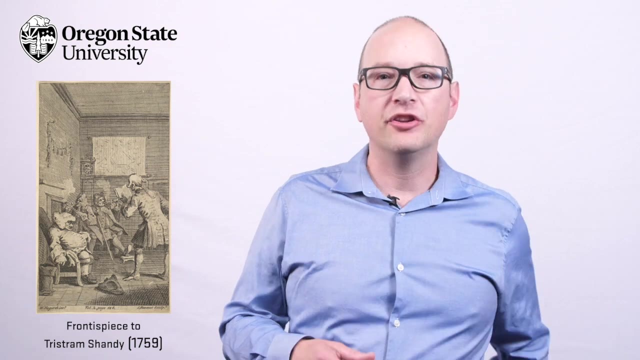 18th-century novel Tristam Shandy, published in nine volumes between 1759 and 1767.. While technically the life story of the eponymous narrator, the novel is far less interested in any kind of linear plot than it is in accumulating incidents and characters and materials that 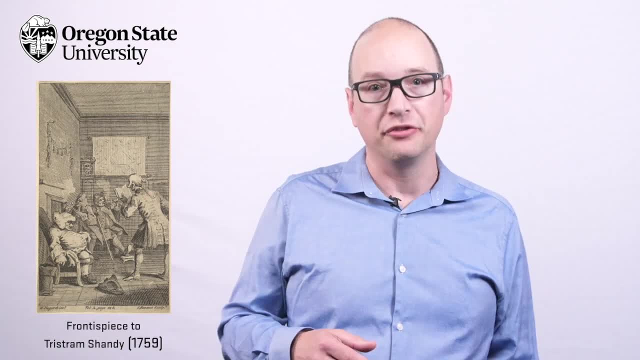 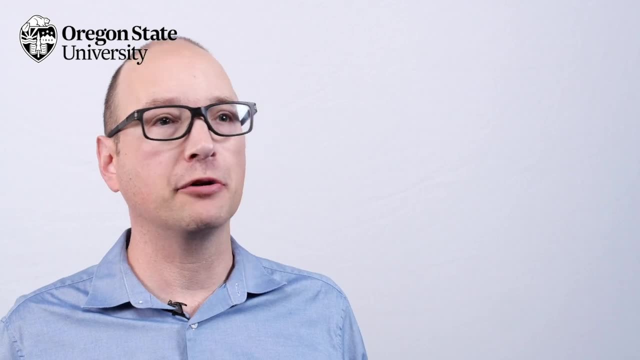 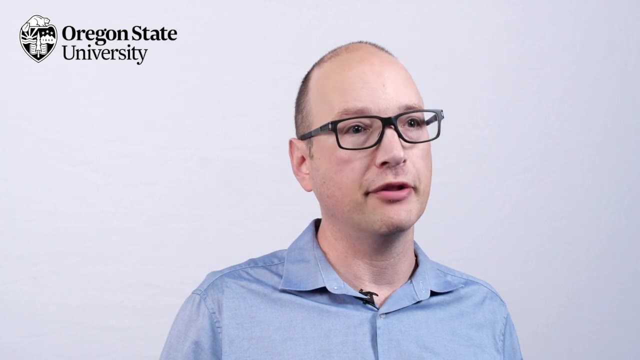 gently molly Manipian satires are relatively rare these days, but many so-called postmodern novels, with their encyclopedic range and fondness for esoteric digression, bear a passing relation to the form, From Thomas Pynchon's Massive Gravity's Rainbow to Zadie Smith's Breakout. 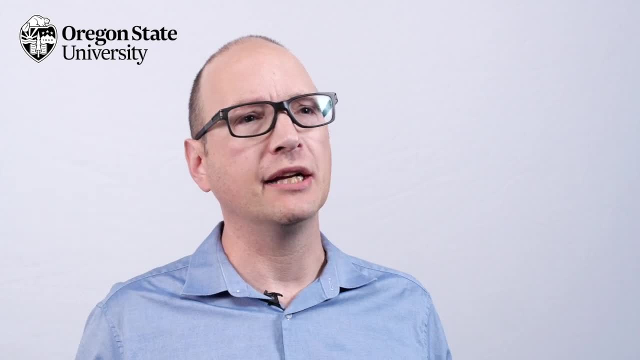 White Teeth. Regardless of which type of satire is being deployed, it must take aim at a target that is larger or more powerful than the original satire. It must be a target that is larger or more powerful than the original satire. Regardless of which type of satire is being deployed, it must take aim at a target that is larger or more powerful than the original satire. 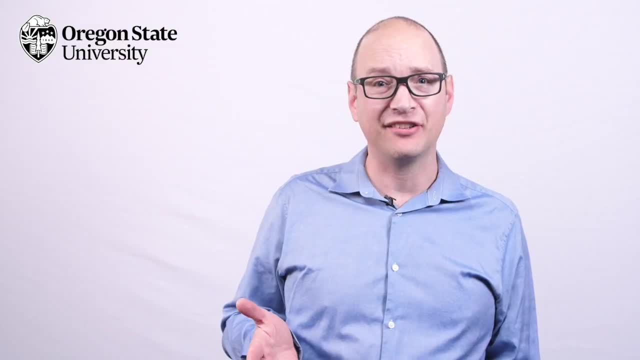 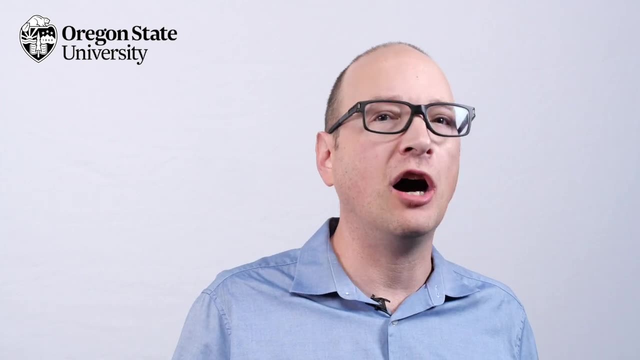 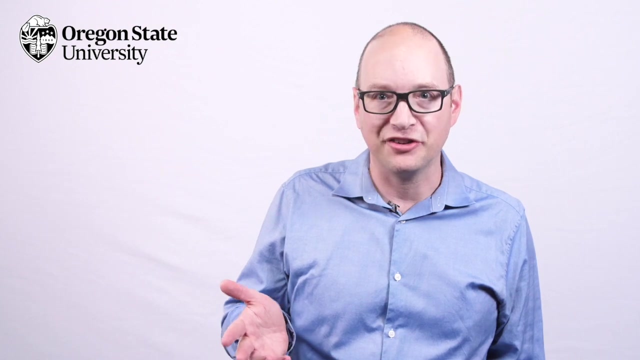 It must be a target that is larger or more powerful than the original satire. Otherwise, instead of satire we have mere cruelty or bullying. So satire is very context-dependent And it also depends on the audience recognizing it as such. For satire to be effective, it must be received as satire. There's always the risk that the satire 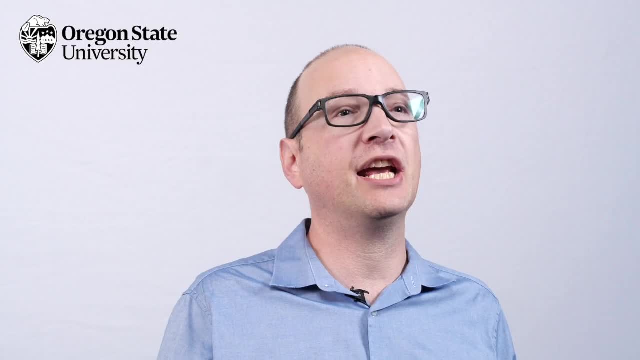 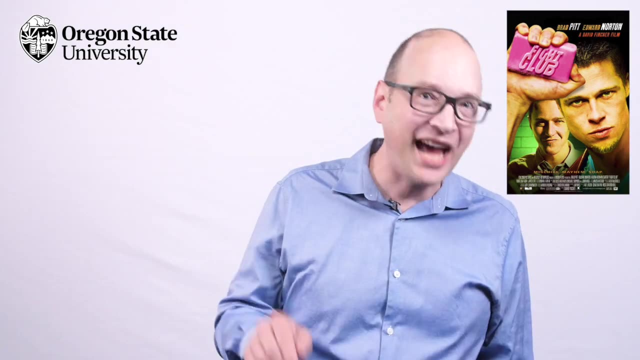 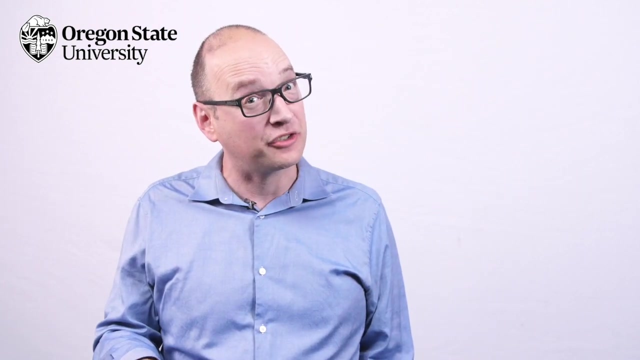 will be read straight or superficially. This was the case, for example, with the reception of David Fincher's 1999 film adaptation of Chuck Palahniuk's novel Fight Club, which satirizes both gender racism and toxic masculinity. Many viewers of the movie apparently didn't understand that it was a satire. 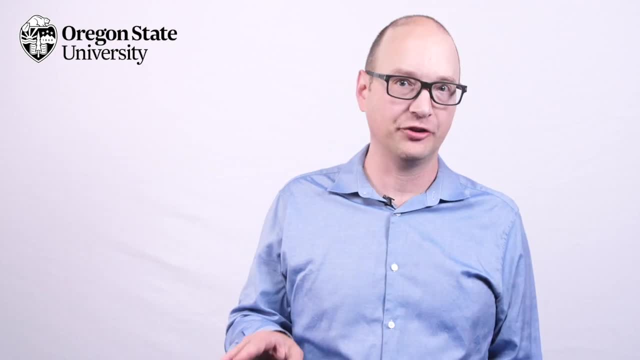 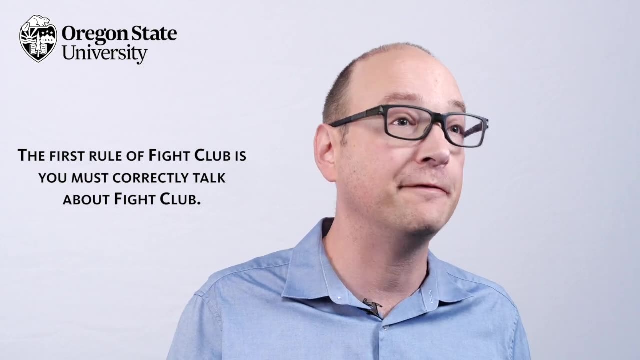 however, since in its wake, a number of real life fight clubs sprung up across the country, Something that shouldn't be happening, had audiences fully understood that the film was making fun of that kind of masculinity that's so desperate to prove itself that it'll happily engage. 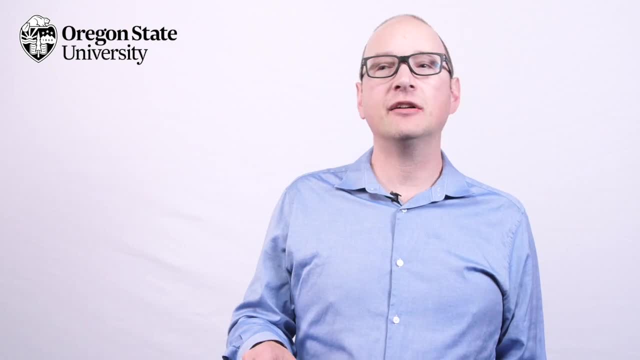 in underground bare-knuckle fighting. Satire is a powerful weapon when it's effectively used and appropriately. Satire is a powerful weapon when it's effectively used and appropriately. Satire is a powerful weapon when it's effectively used and appropriately used. Satire is a powerful weapon when it's effectively used and appropriately used. But it's also a risky weapon when it's effectively used, and gain or lose can also be used if it's sche stroll over and over. So satire isn't always as risky as the actual crime in America, but satire and religious Lynnerei will still have better. 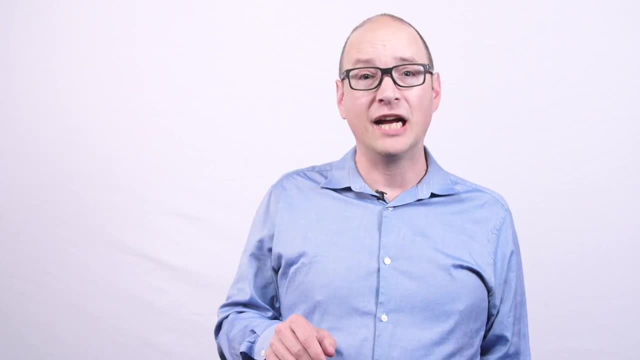 But it's also a risky one too, which is probably a big reason why it remains so fascinating for authors and audiences alike.